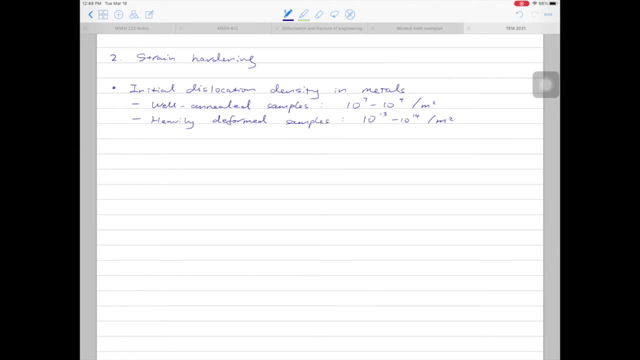 to 10, to the 14th per meter square. There are a couple of notes I'd like to make here. When we compare the dislocation densities, we usually don't care about the exact numbers. What we worry about are the orders of magnitudes. 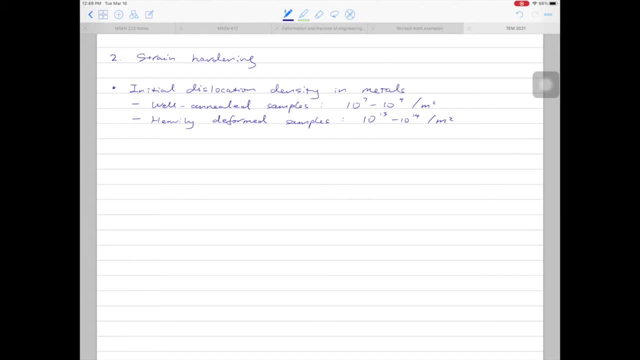 For example, 10 to the 7 versus 10 to the 13.. Second, let's look at the unit of dislocation density. The unit is per meter square. The reason is because dislocation density is dislocation length divided by volume. The length unit is meter, The volume unit is meter cube, Meter over meter cube. 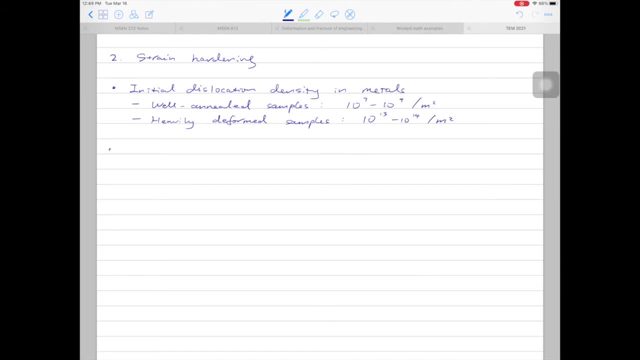 gives us per meter square. Next, let's look at the deformation behavior of single crystals, especially those aligned to encourage single slip. Here is the shear stress versus shear strain plot. The initial part is linear, elastic. Further straining the sample will activate dislocations and we enter plastic regime. 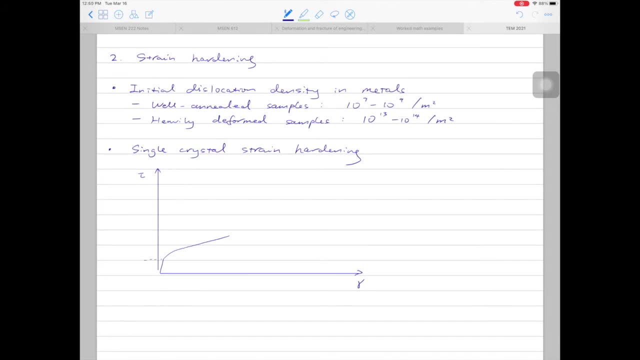 At the transition of elastic deformation and the plastic deformation. we can easily identify the CRSS, CRSS, CRSS, CRSS specimen. you will see the first dramatic change in the strain hardening rate and as the deformation proceeds you will see another change. Depends on the strain hardening rate the plastic regime can. 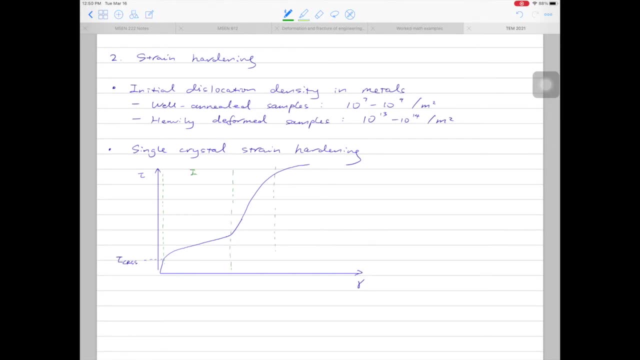 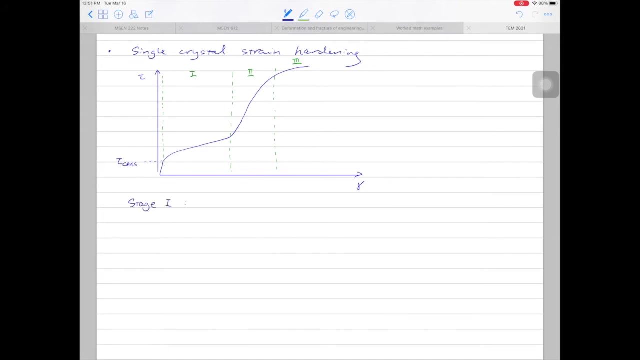 be divided into three stages. These are called stage 1, stage 2, and stage 3.. The question is what kind of dislocation behavior lead to these three distinct stages? For stage one, as you can see, the strain hardening is fairly low. in this stage, Dislocations can easily glide and multiply. 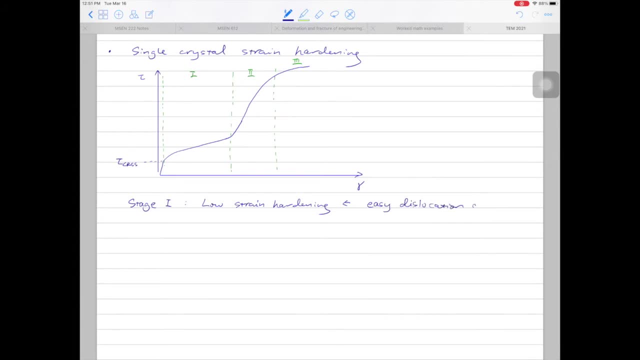 in the crystal without too much interaction. that's why we don't get too much strain hardening in this stage. In stage 2, there is a dramatic increase in the strain hardening rate, indicated by a rapid increase in the saitening rate. Can you see the difference? It's enormous. 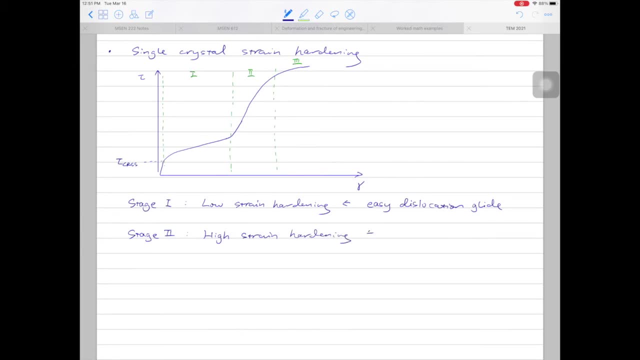 increase in stress at given strain. At this stage dislocations start to interact with each other, to form dislocation entanglements. One example is something we have already covered in one of the previous videos: the quadrilateral locks. In the quadrilateral locks we start by two sessile dislocations, gliding on two different 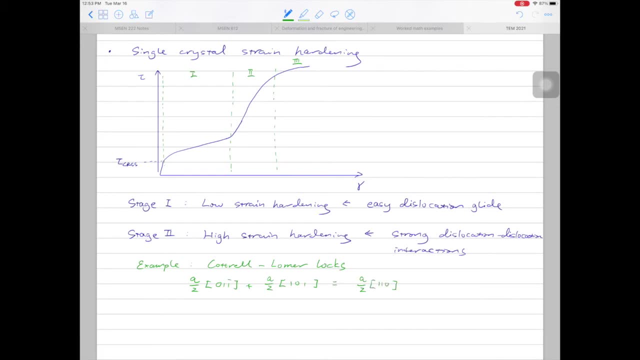 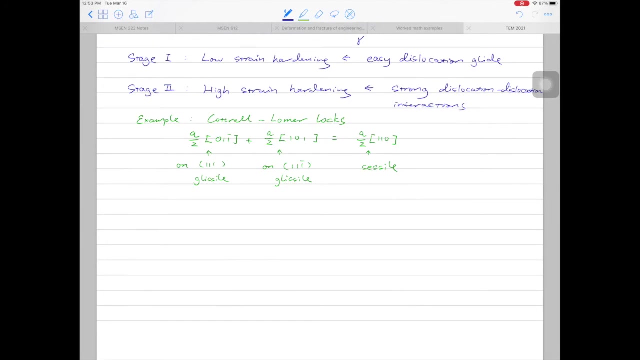 planes. then they meet at one point and form a sessile lock. These quadrilateral locks can behave as dislocation barriers for dislocation glide, leading to the strong strain hardening With further plastic deformation. we'll enter stage 3.. We have learned that when the dislocation 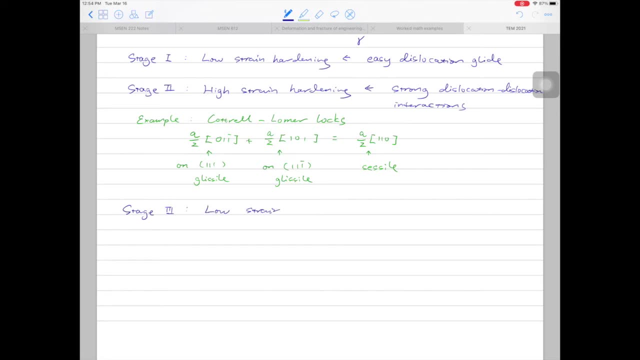 density in the material is extremely high. such a configuration is not thermodynamically stable. Any thermal perturbation, even room temperature, can help dislocations to rearrange, to reduce the overall strain energy. The result is something we call dynamic recovery At the microstructure. 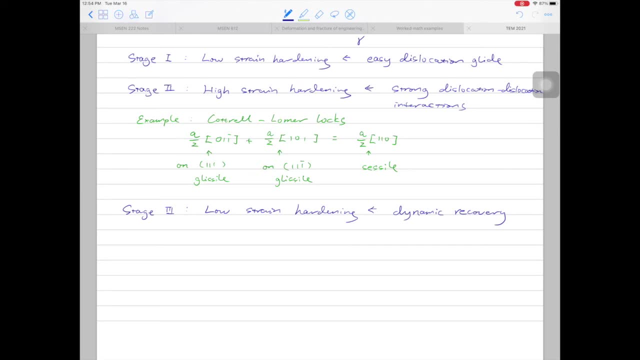 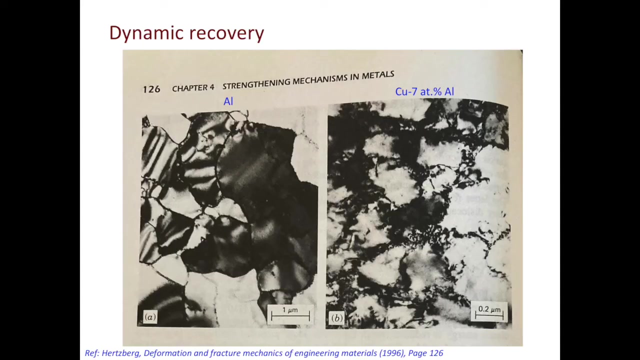 and dislocation level. what's going to happen is those dislocations will rearrange themselves to form sub-grain boundaries or dislocation arrays. In this stage, the strain hardening rate will decrease a lot. Here are two examples showing the dynamically recovered microstructure in aluminum and copper-aluminum. 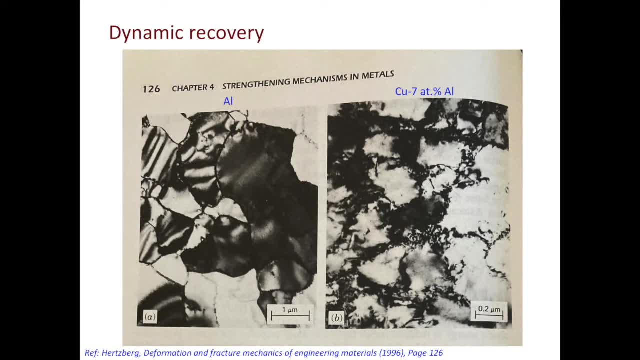 alloy. In both cases the dislocations rearranged themselves to form cell boundaries, and within each cell there's nearly no dislocations. One interesting observation to make is that the cell boundaries in aluminum seem to be sharper than the ones in the copper alloy. 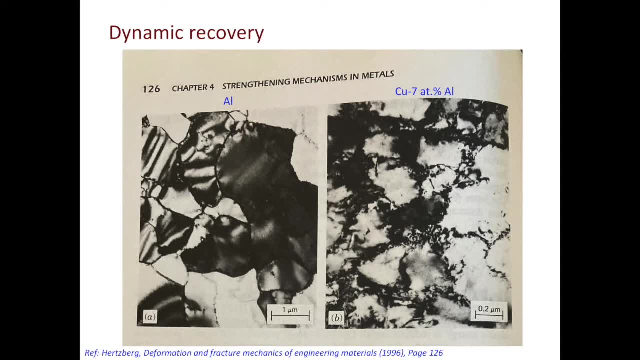 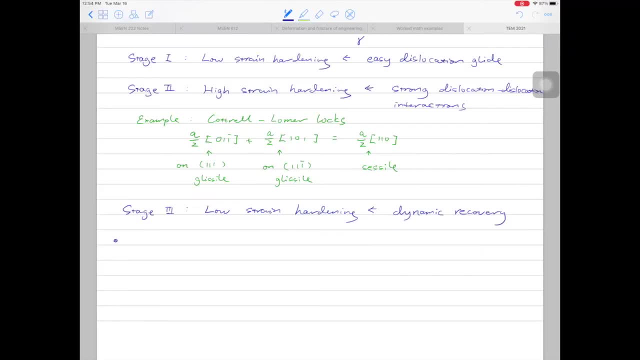 This difference is caused by the dynamic recovery of the microstructure in aluminum and copper-aluminum. As you can see in the picture below, the bounce in microutlich is felt from the mattex deposit on the öldre alloys, but the